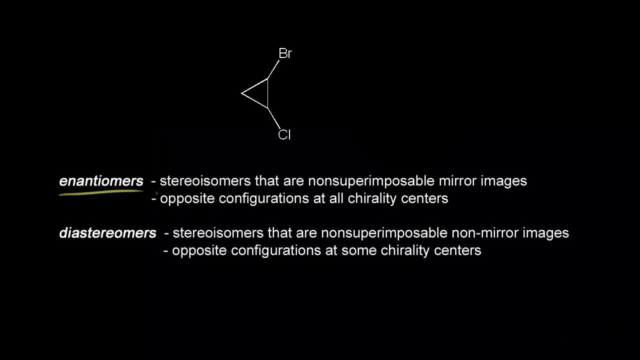 We've already spent a lot of time talking about enantiomers. These are stereoisomers that are non-superimposable mirror images of each other And they have opposite configurations at all chirality centers. Diastereomers are also stereoisomers. 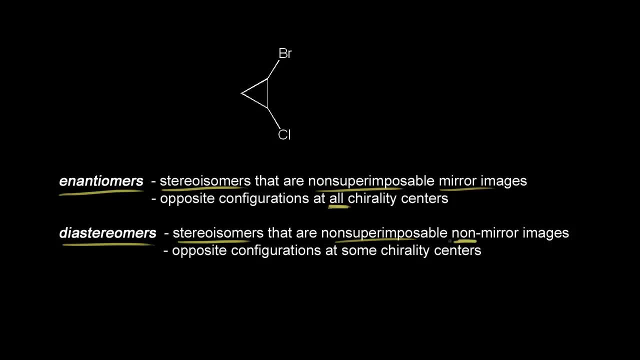 but these are stereoisomers that are non-superimposable, non-mirror images of each other. So these are stereoisomers that are not enantiomers And diastereomers have opposite configurations at some chirality centers, If we look at this compound up here. 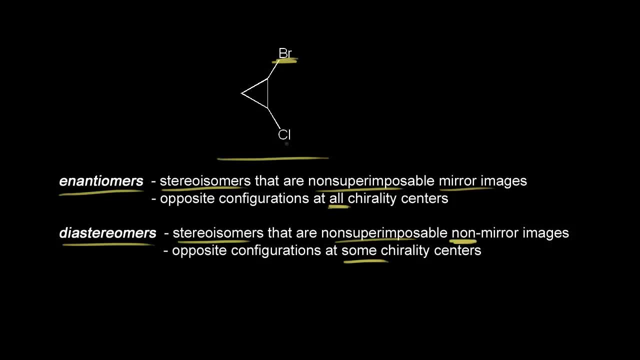 we have a cyclopropane ring with a bromine coming off and a chlorine coming off. We know from earlier videos that there are two chirality centers, So this carbon is a chiral center and so is this one. The total number of stereoisomers is two to the n. 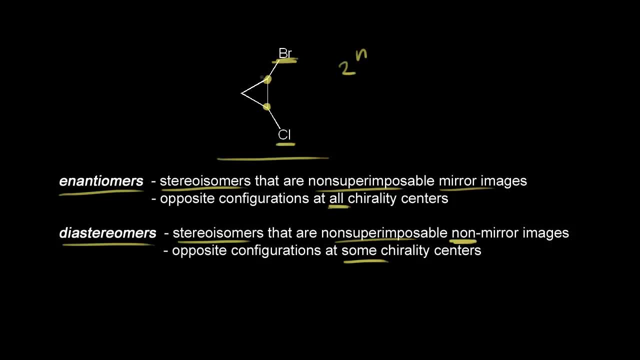 where n is equal to the number of chiral centers. And since n is equal to two, for this drawing we would expect to be able to draw two to the second power or four stereoisomers, So there should be a total of four stereoisomers. 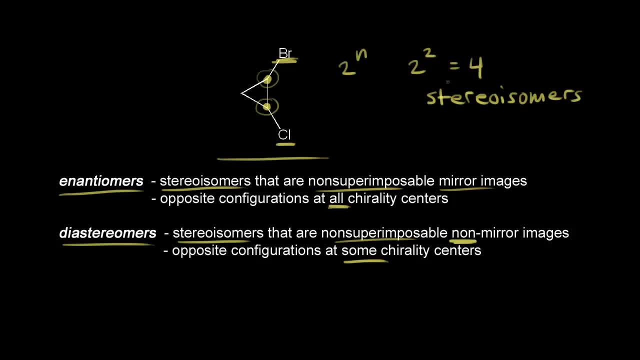 Actually, two to the n is just a maximum and we'll talk about that in later videos. So let's draw all four stereoisomers and let's look at the relationship between them. Let's think about how to draw our four stereoisomers. 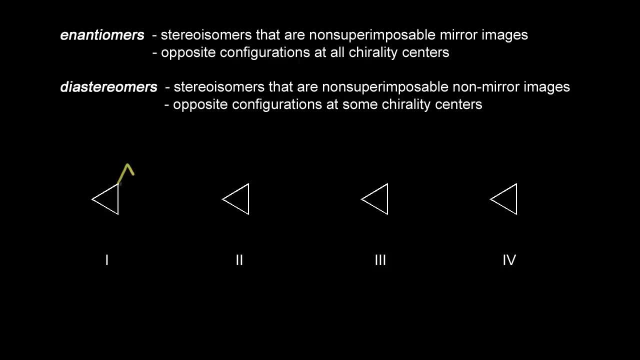 For the first one, we could have both halogens coming out at us in space. So I put the bromine on a wedge and I put the chlorine on a wedge. Next, we could have both halogens going away from us in space. 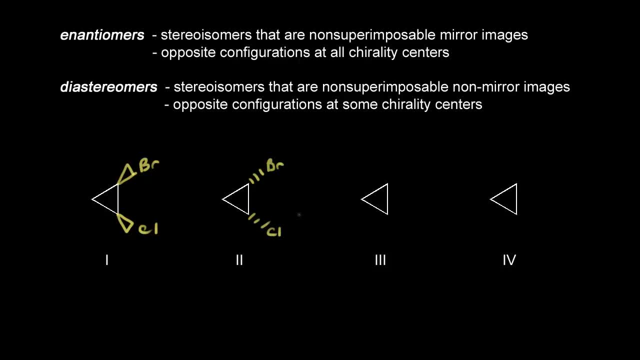 So I put the bromine on a dash and same with the chlorine. Next, for our third stereoisomer, we could have one halogen coming out at us, So I'll make that the bromine and one going away from us, And for the last one we could just reverse it. 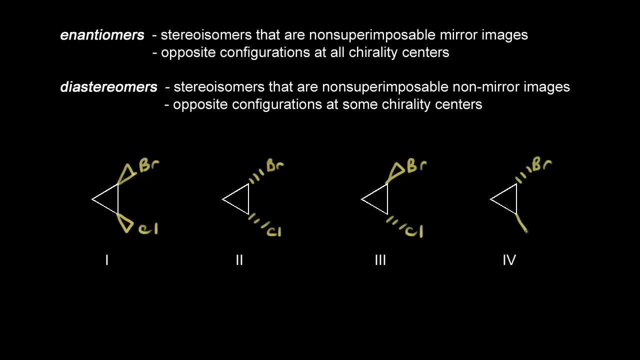 We could have the bromine going away from us and the chlorine coming out at us. Next, let's look at the relationships between our stereoisomers, And let's start with the relationship between stereoisomer one and stereoisomer two. Model sets really help in stereochemistry. 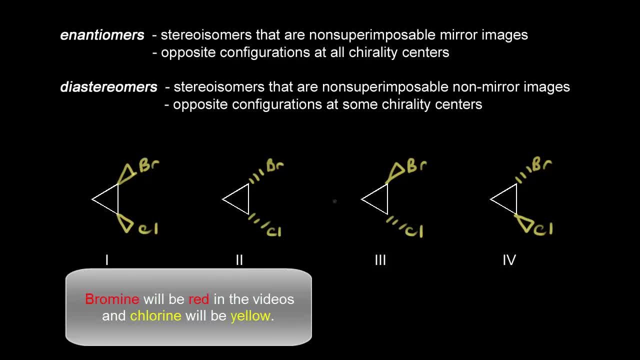 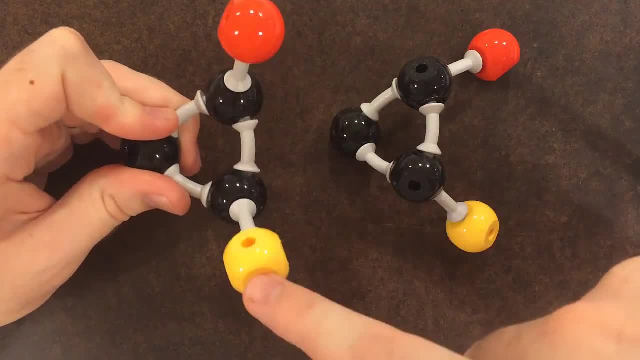 so we're gonna look at videos for a lot of these. Let's look at the video comparing stereoisomer one and stereoisomer two. On the left we have stereoisomer one. Both halogens are coming out at us in space. 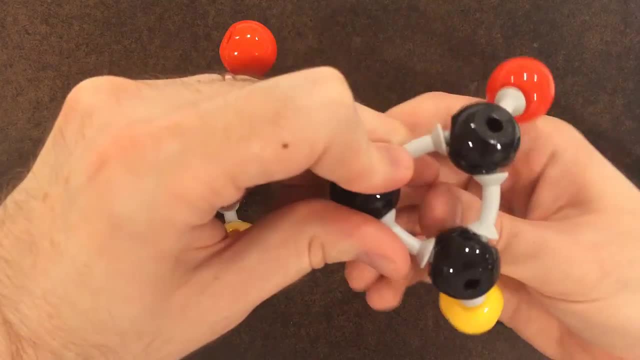 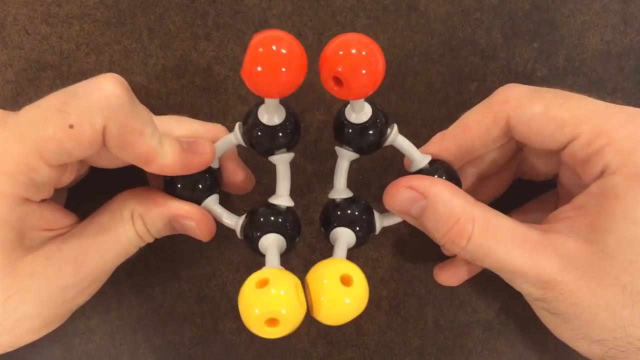 On the right is stereoisomer two, where both halogens are going away from us in space. If I hold these two stereoisomers next to each other and I rotate the one on the right, we can see they're actually mirror images of each other. 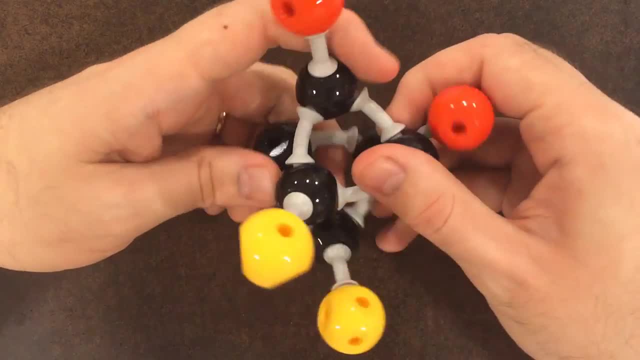 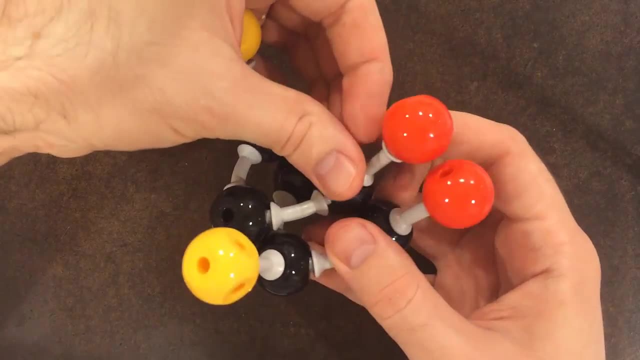 And they're non-superimposable mirror images. If I line up the chlorines, then the bromines are not in the right position, And if I try to line up the bromines now, the chlorines are not in the right position. 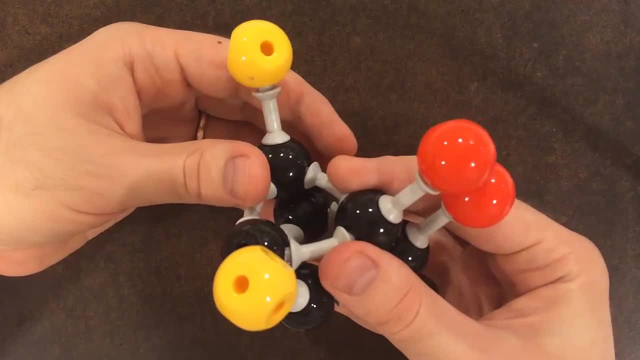 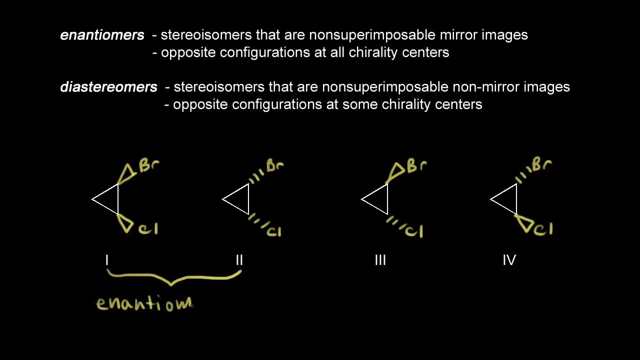 So these are non-superimposable mirror images of each other. These are enantiomers. So we saw in the video that one and two are enantiomers of each other. They are non-superimposable mirror images And they have opposite configurations. 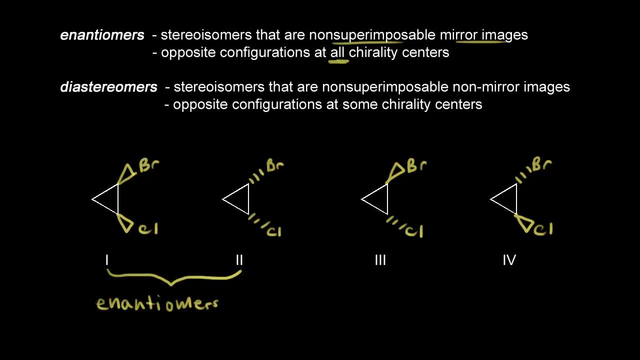 at all chirality centers, And that's easy to see if you look at the drawings here. So at this carbon we have bromine on a wedge And if we change it to a dash, we see we have this one on the right. 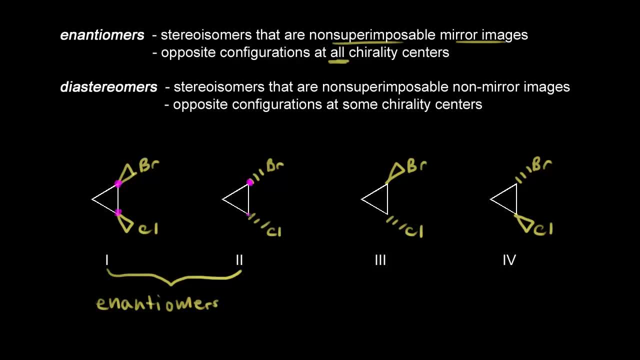 If we look at this chiral center, we have chlorine on a wedge, And here it's changed to a dash. So that's an opposite configuration at both chiral centers, And so that's how we know. that's one way of knowing that this one on the right is the mirror image. 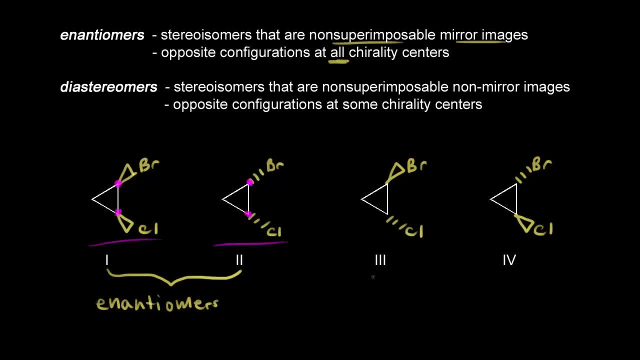 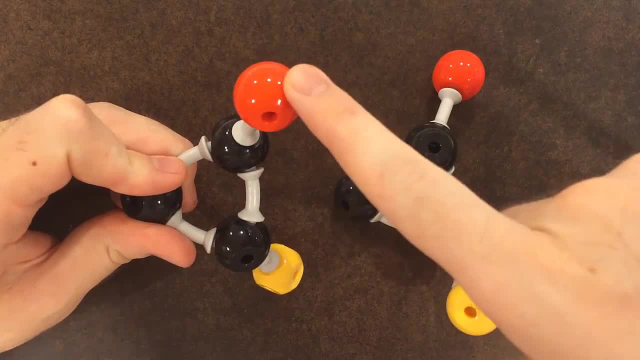 of the one on the left. They are enantiomers. Let's look at the relationship between stereoisomers three and four. On the left is stereoisomer three with bromine up and chlorine down. On the right is four with bromine down and chlorine up. 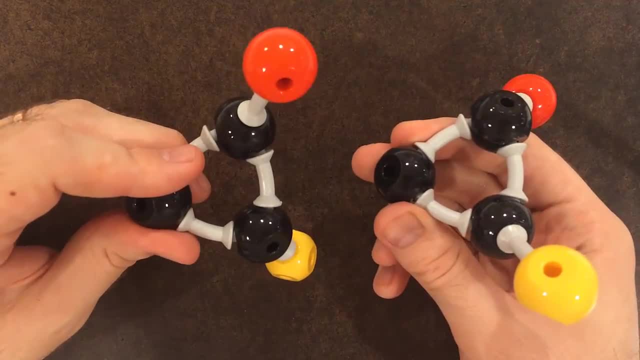 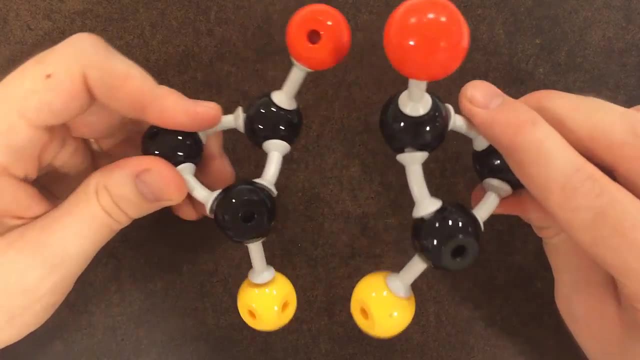 If we hold them together and I rotate the one on the right, it's easy to see that these are mirror images of each other And they are non-superimposable. If I put the chlorines on top of each other now, the bromines don't line up. 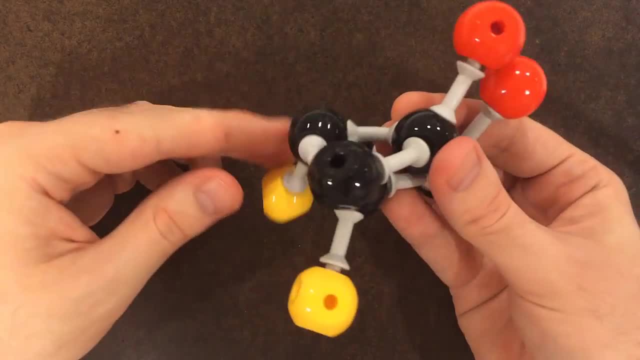 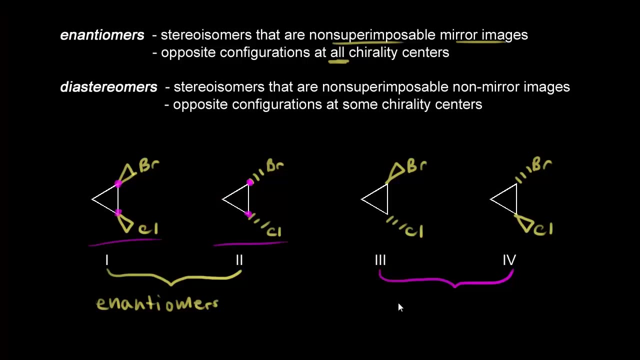 And if I try to line up the bromines then the chlorines don't. So these are non-superimposable mirror images of each other. These are enantiomers. So three and four are enantiomers of each other. They are non-superimposable mirror images. 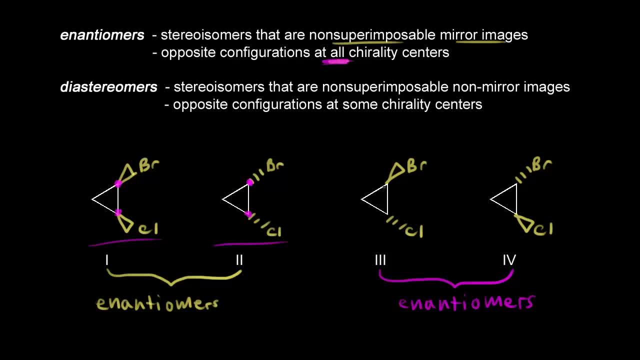 And they have opposite configurations at all chirality centers. So at this chiral center we have, for example, here we have bromine on a wedge, and over here we have bromine on a dash. At this chiral center we have chlorine on a dash. 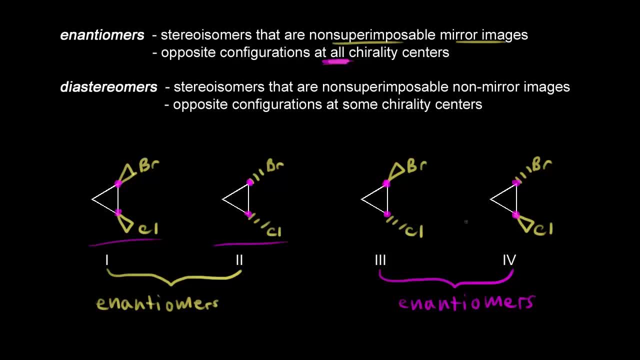 and over. here we have it on a wedge, So we have opposite configurations at both chirality centers. Next let's compare stereoisomers two and three. So what's the relationship between two and three? On the left is stereoisomer two. 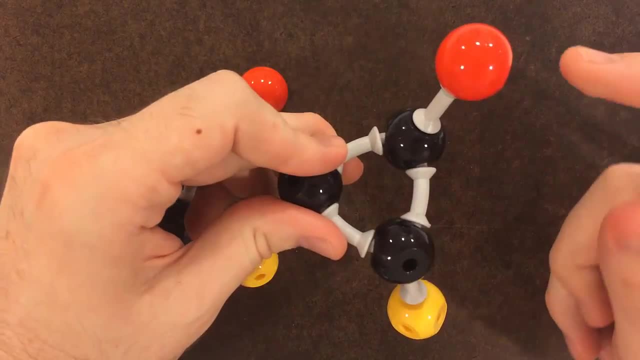 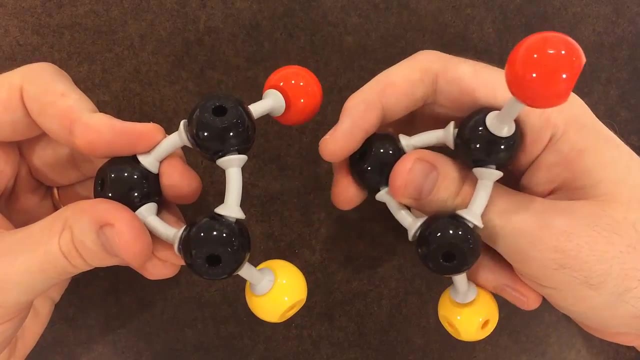 with the bromine and the chlorine going away from us in space. On the right is three, with bromine up and chlorine down. If I hold the two stereoisomers next to each other and I rotate the one on the right, we can see these are not mirror images of each other. 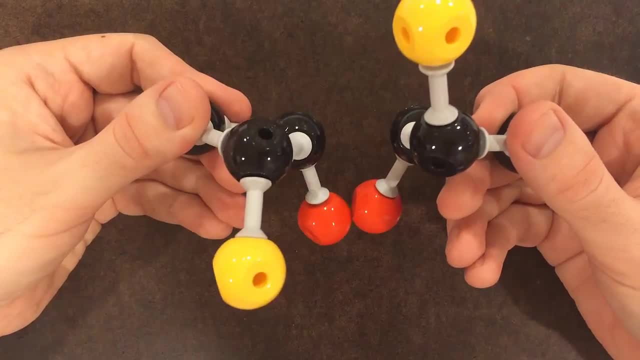 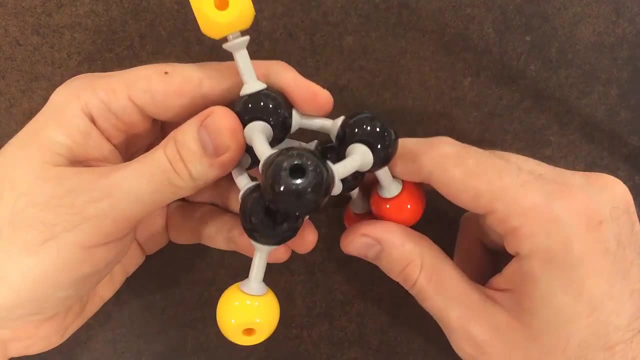 The bromines look right, but the chlorines don't. One chlorine is up and one chlorine is down. If I try to superimpose these, I can get the bromines to match but not the chlorines. And if I try to make the chlorines line up, 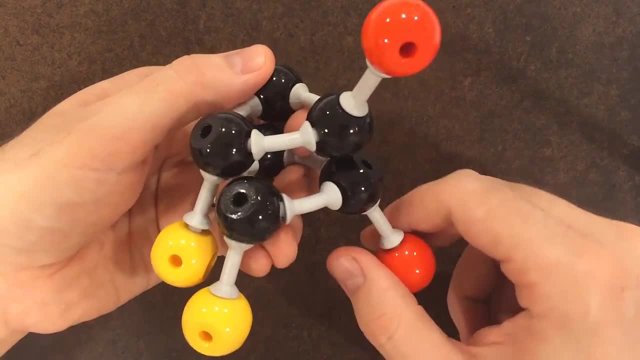 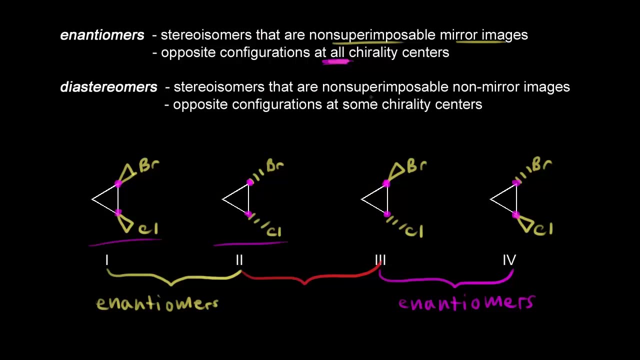 then the bromines won't. So these are non-superimposable, non-mirror images. These are diastereomers. We saw in the video that two and three are non-superimposable and they're also non-mirror images. 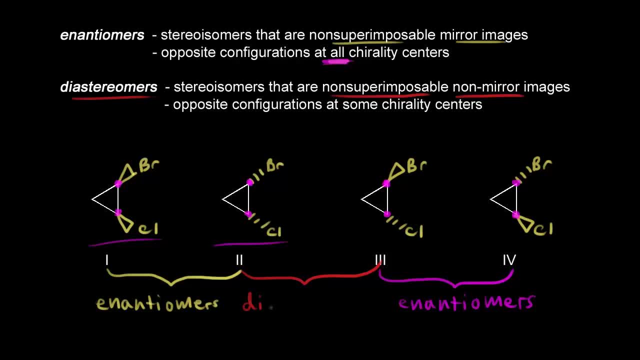 Therefore they are diastereomers. Let me write that down here. So two and three represent a pair of diastereomers, And diastereomers have opposite configurations at some chirality centers. So if we look at this, carbon, 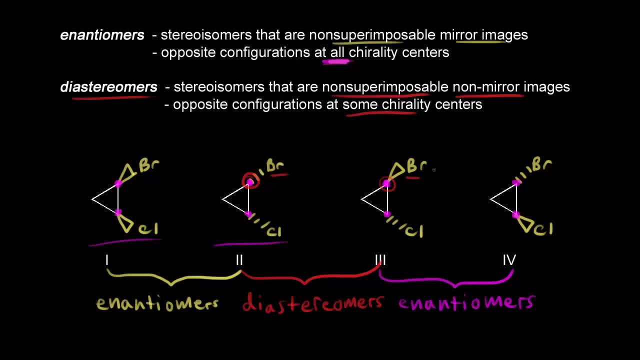 we have bromine on a dash and over here we have bromine on a wedge, So that's opposite. But if we look at this one, we have chlorine on a dash and over here we have chlorine on a dash, So that's the same. 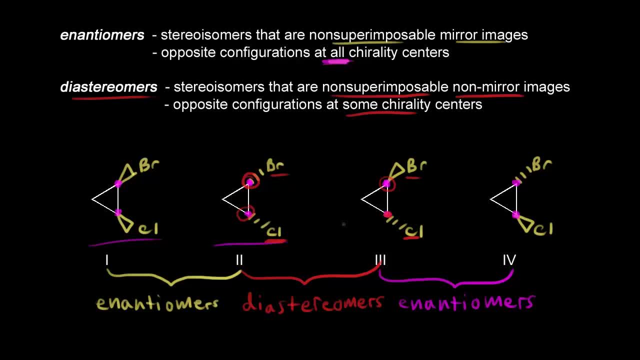 So we only have an opposite configuration at one chiral center, And so these are diastereomers. What about comparing two, stereoisomer two, with stereoisomer four? So let's look at the video, for that. On the left is stereoisomer two. 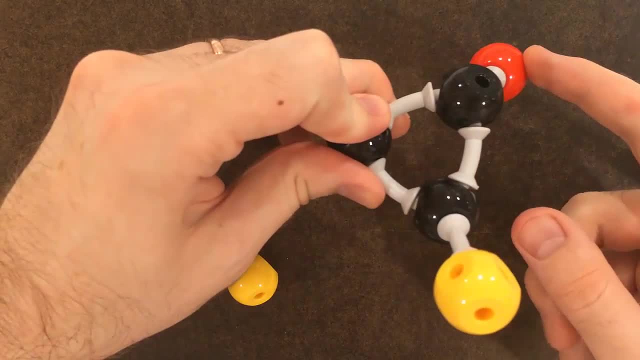 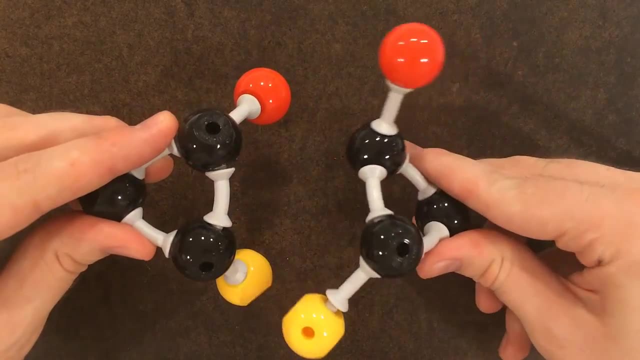 with the bromine and chlorine going away from us On the right is four, with bromine down and chlorine up. So we hold the two stereoisomers next to each other and we rotate the one on the right And we can see these are not mirror images.